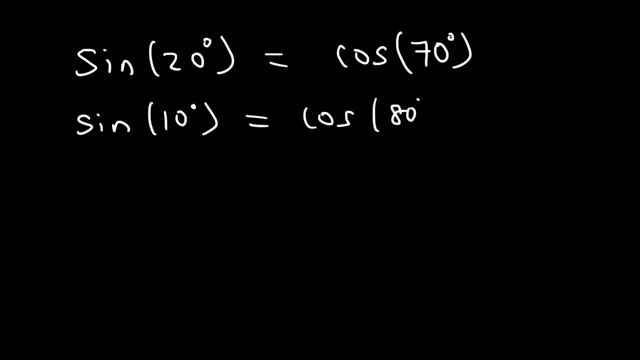 is equal to cosine 80, because 10 plus 80 adds up to 90, sine 0, for example, is equal to cosine 90. Both sine 0 and cosine 90 is equal to 0. And sine 45 is equal to cosine 45, which both of them are equal to the square. 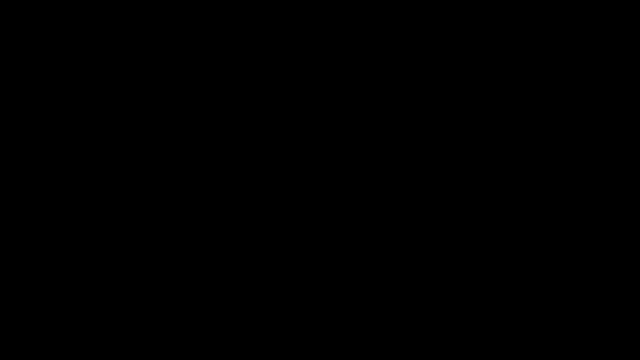 root of 2 over 2.. So what I'm going to do is I'm going to give you some practice problems and I want you to identify the co-function with the appropriate angle. So try this one: Sine, 65 degrees tangent 20 degrees cotangent pi divided by 3, secant 42, and also cosine. 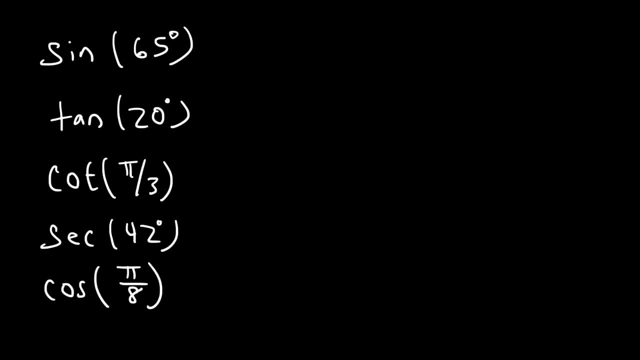 of, let's say, pi over 8.. So, starting with the first one, The co-function of sine is cosine. So this is going to be cosine 90 minus 65. And 90 minus 65 is 25.. So that's the answer for the first one. So sine 65 is equal to cosine 25.. 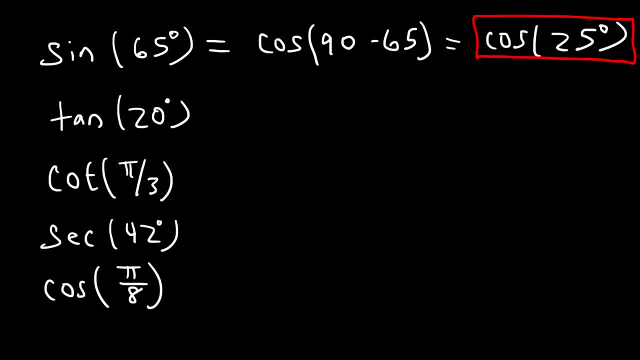 Now what about the second example, Tangent of 20 degrees. What's the co-function of tangent? The co-function of tangent is cotangent, And so this is going to be cotangent 90 minus 20, which is 70 degrees. So the answer is: 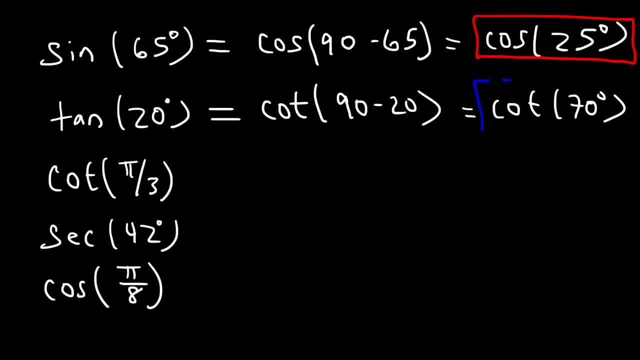 cotangent 70 degrees. That's the co-function of tan. Now what about cotangent pi over 3?? Well, the co-function of cotangent is tangent And instead of being 90 minus an angle in degrees, 90 is pi over 2 in radians. So it's going to 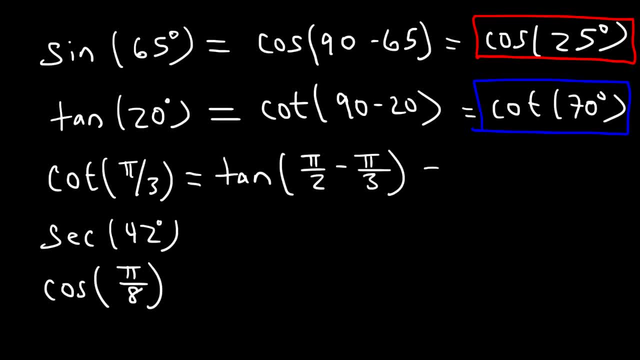 be pi over 2, minus pi over 3.. So what we need to do is get common denominators. I'm going to multiply this fraction by 3 over 3.. So it becomes 3 pi over 6.. And this one I'm going to multiply by 2 over 2.. So it becomes: